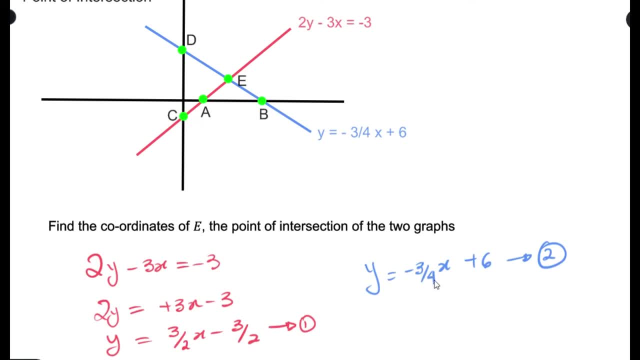 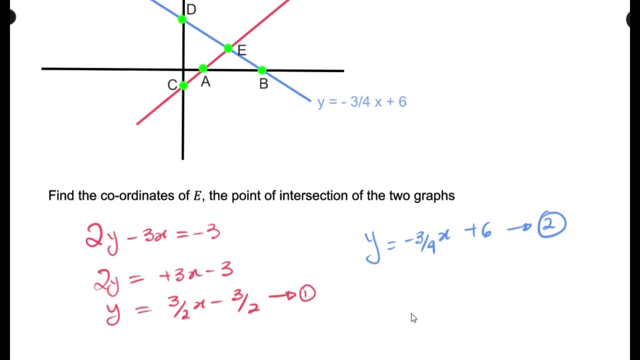 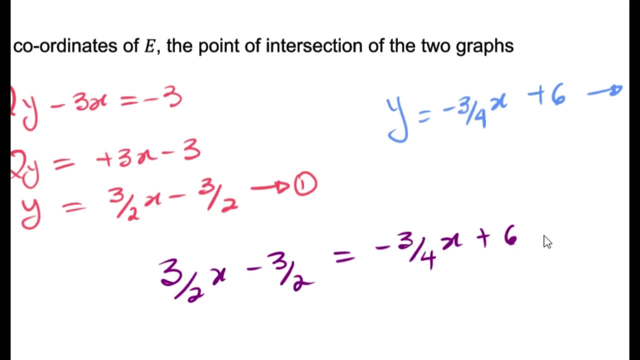 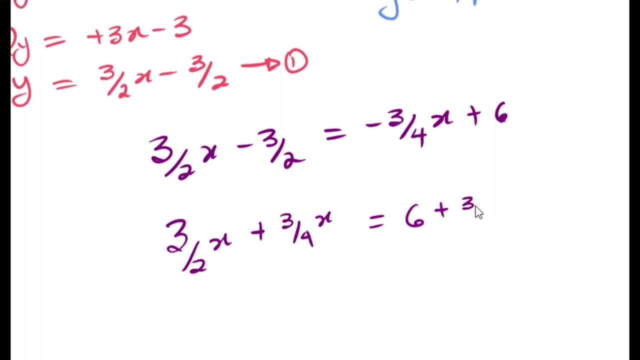 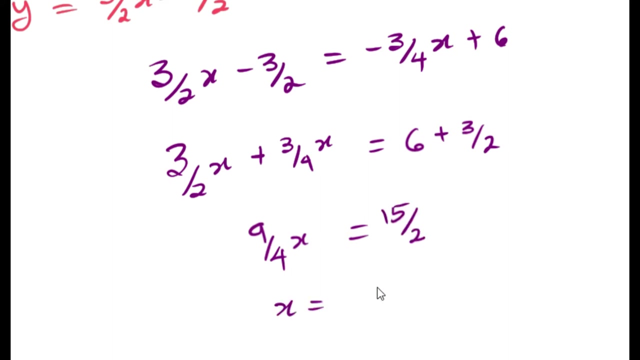 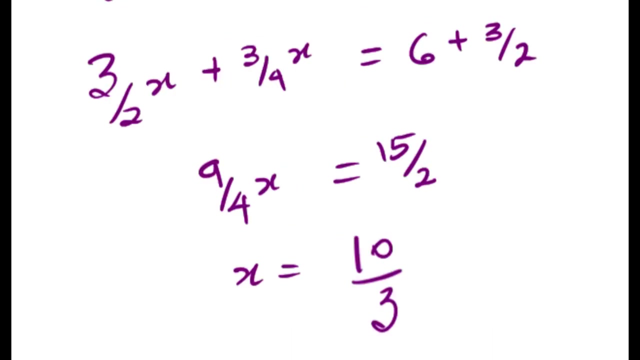 plus 3 over 2 for the first equation, and Y is equal to negative 3 over 4X plus 6 for the second equation. we can just equate both equations, right? We see that we simplified. Now this is your x coordinate. To get the y coordinate, we just need to substitute this: 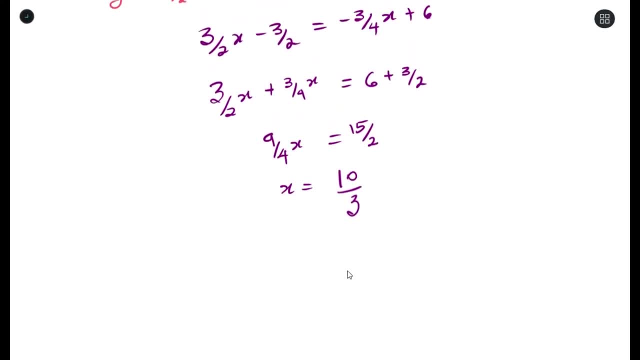 value for x into any of the two equations. So, substituting you would get: the coordinate of your point of intersection would be 10 over 3 and 7 over 2.. So that's your value for E And that's it.